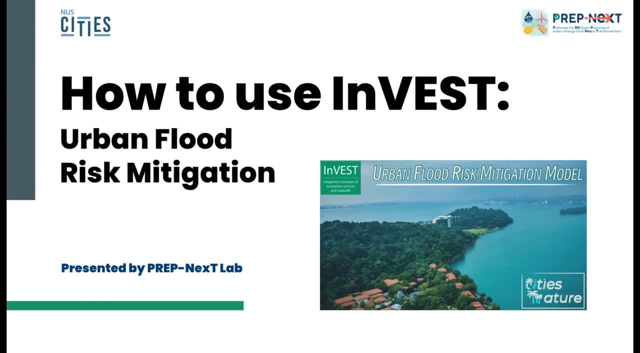 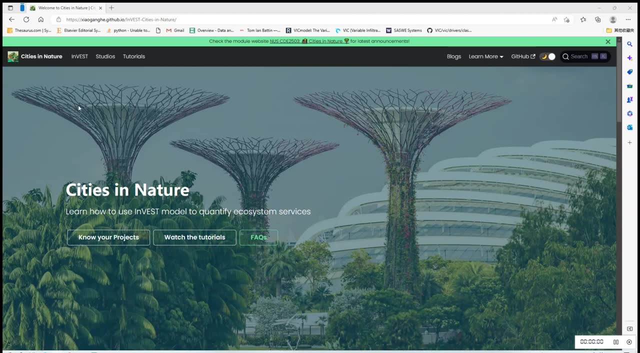 Hello everyone, in this video we'll be showing how to use the INVEST Urban Flood Risk Mitigation Model. Similar to other models, we need to first navigate to the Cities in Nature homepage and find the INVEST button on top. Click INVEST and the introduction of INVEST and the details. 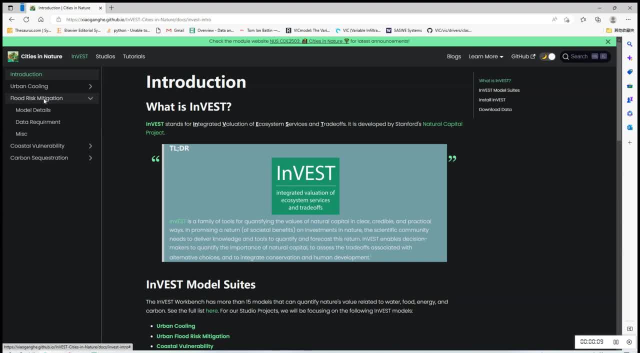 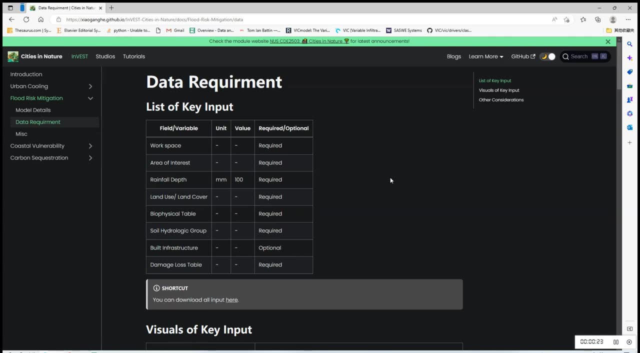 of the four models will appear In this video. we are showing you how to use the Urban Flood Risk Mitigation Model. So click data requirement for this model and you'll see a list of key input that is required to run the model. These data can be downloaded by clicking the link. 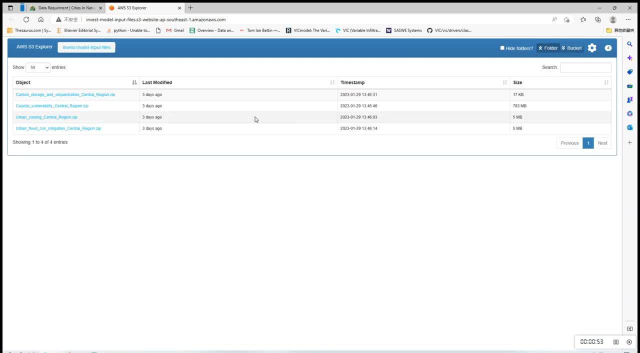 below. In this case, let's download the Urban Flood Risk Mitigation file. The files we are using in this demo video are for the Central region, only For Central area and Queenstown. you'll need to download the other corresponding files. Click to download and you'll see there are. 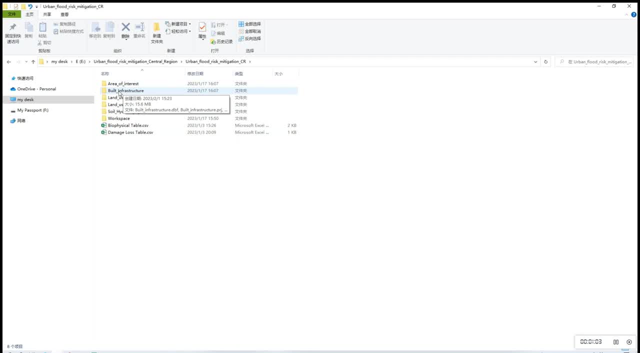 multiple files under the zip folder. Remember to extract all files before uploading them into INVEST, otherwise the model won't work. The names of these folders correspond to the name of the entries inside INVEST. So now let's open up INVEST. 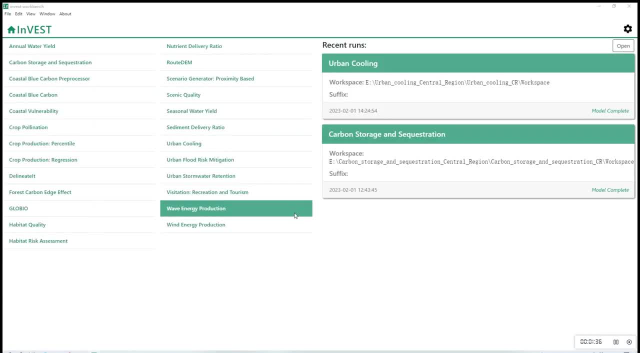 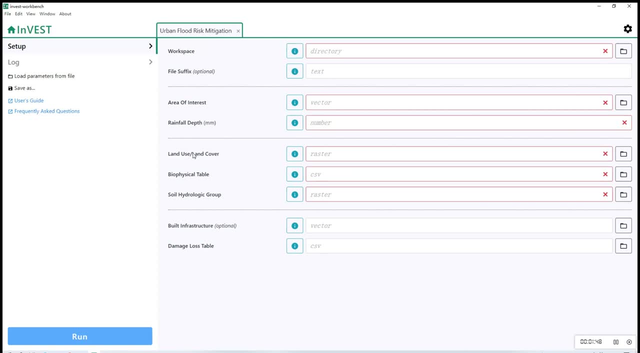 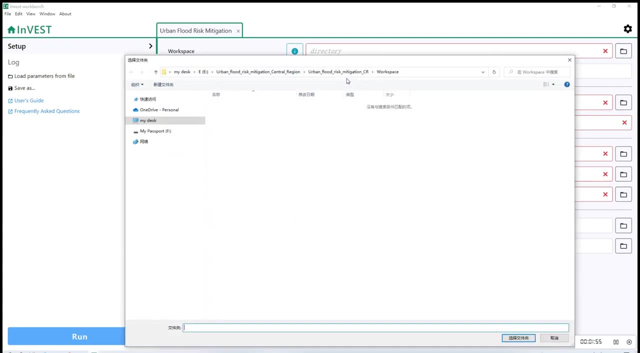 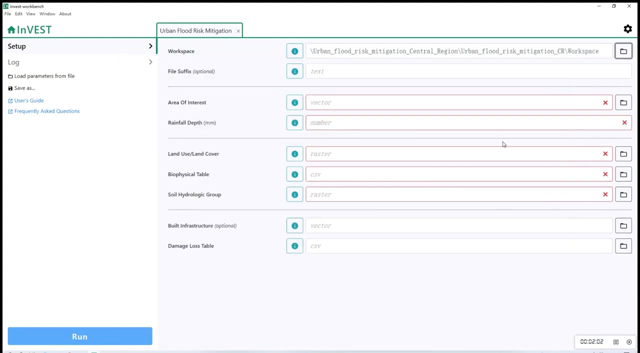 So now let's open up INVEST. Click the Urban Flood Risk Mitigation Model and you'll see all the entries here We can start uploading the files into INVEST. Click the folder icon. This entry is workspace, so we need to find the folder that is named as workspace and upload Similarly for area. 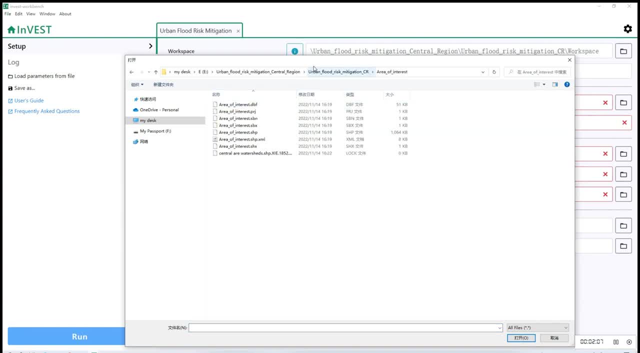 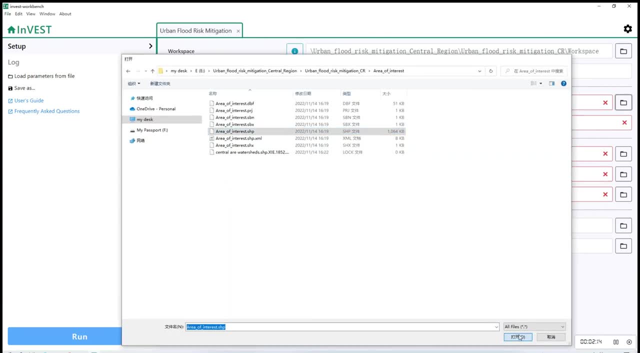 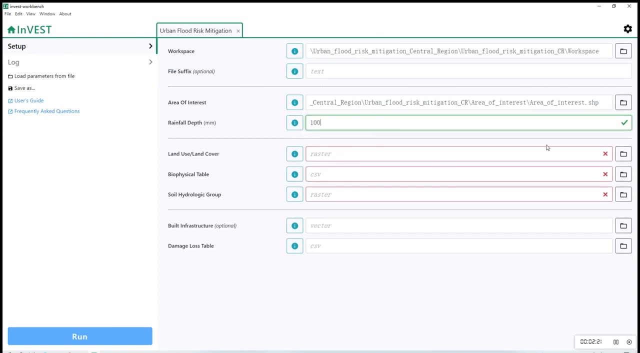 of interest. you'll find the folder named workspace And here you need the file that is in the format of SHP. For rainfall depth, if you recall from the data requirement table, it should be 100.. For land use: land cover: choose. 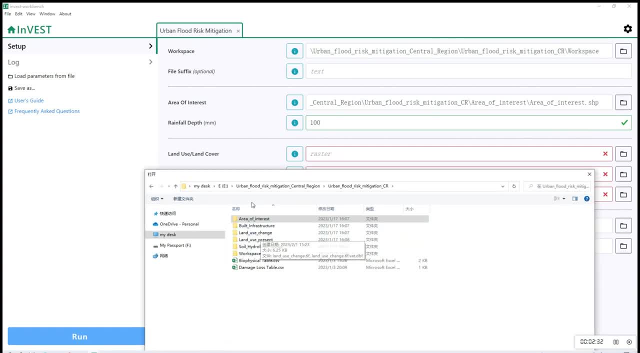 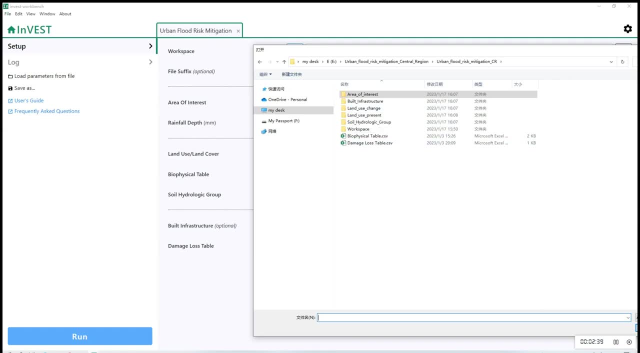 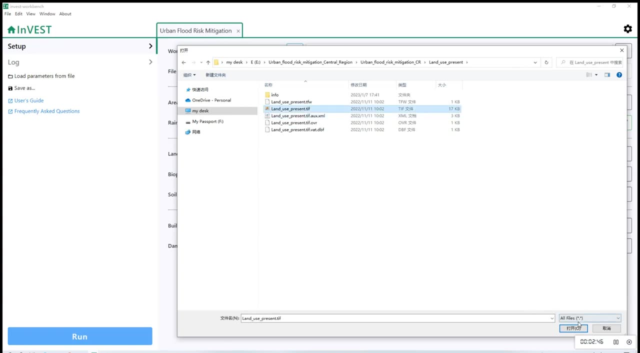 land use present or change. So if you choose land use present, there is a file in the format of TIFF. So choose the TIFF file And if you choose land use change, similarly you can choose the TIFF file as well. For biophysical table: choose the file that is in the format of CSV. 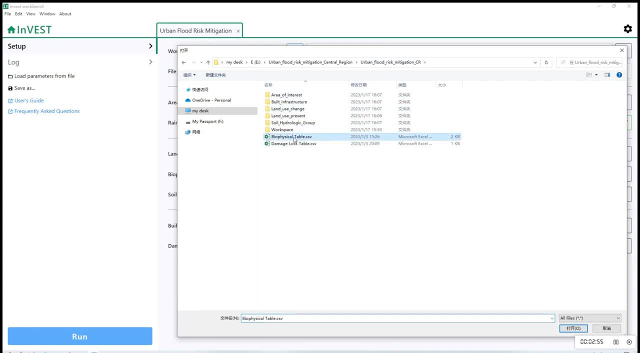 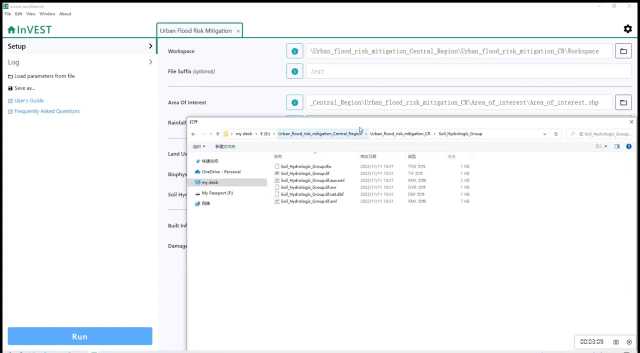 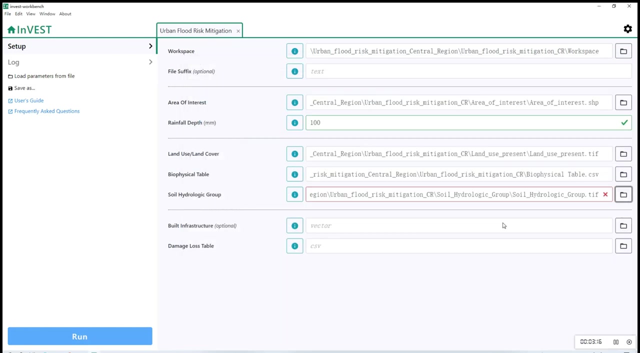 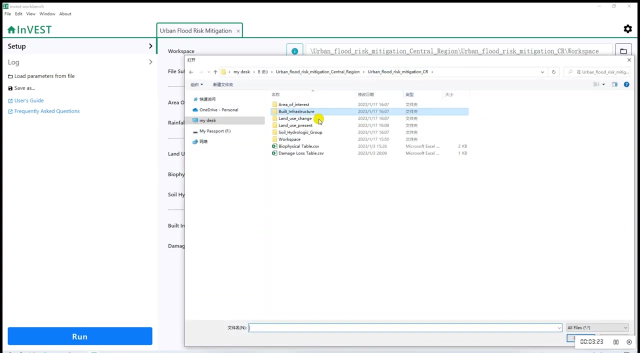 and repeat the steps for the rest of the data entries. For soil hydrologic group: open the soil hydrologic group folder and there is a TIFF file that you should upload to INVEST. Choose the second file and upload For built infrastructure: similarly, there is a folder called built infrastructure And the file that you 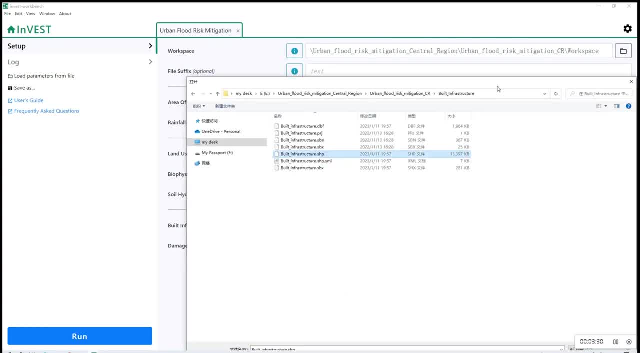 should be uploading is the file in the format of SHP. And lastly, there is a damage loss table, which is an impact operation. We go in the FHA case as well today and fill out here And then we go into and the child data too. And then we're when you go filig за data entry, you need to follow the last role that we're consecutively given, one to follow as the file, So that they're often forgotten. And then we go back to localed beliefs in these previous videos to spice things up. 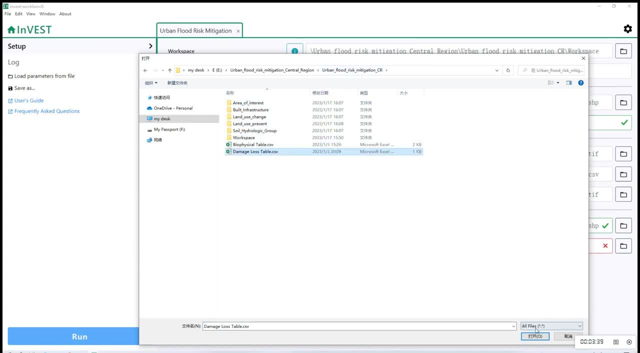 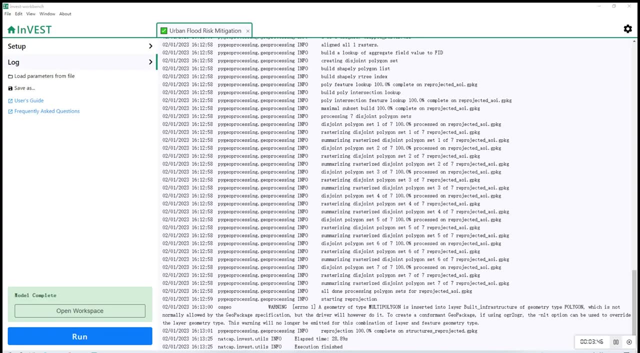 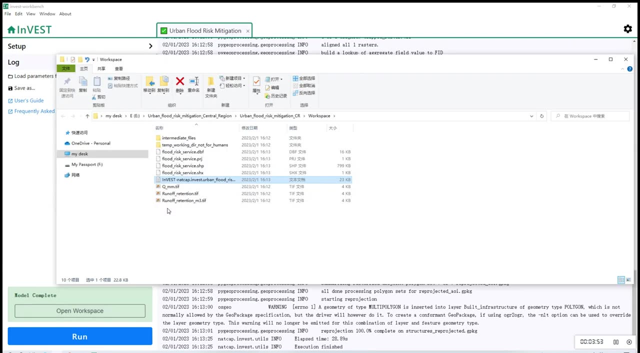 As you can see, and you can just press the volume and then drag it from the. the common is in the format of csv. Upload this file and you are ready to run. Run the model and once it's complete it will show the model is complete and you can open workspace and all the output files. 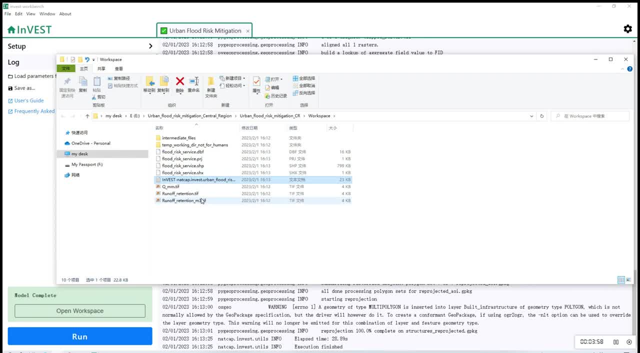 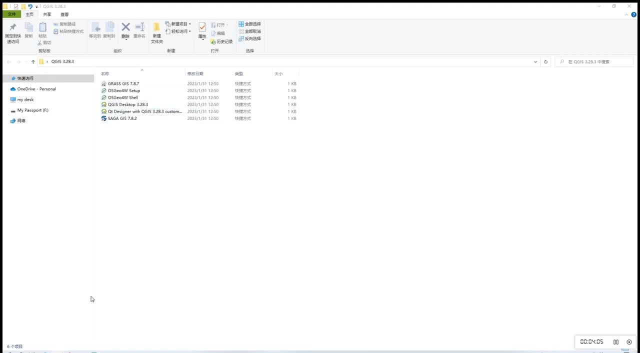 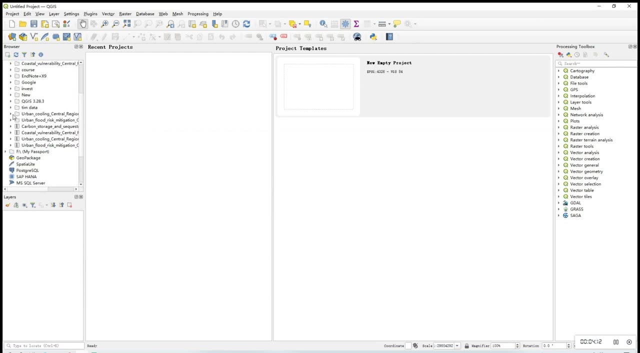 will be here under your workspace folder. So in order to view these images, you need to download QGIS and open QGIS. So the files will be under urban flood risk mitigation folder and find your workspace folder. Under the workspace folder there will be some tiff files which are your outputs. 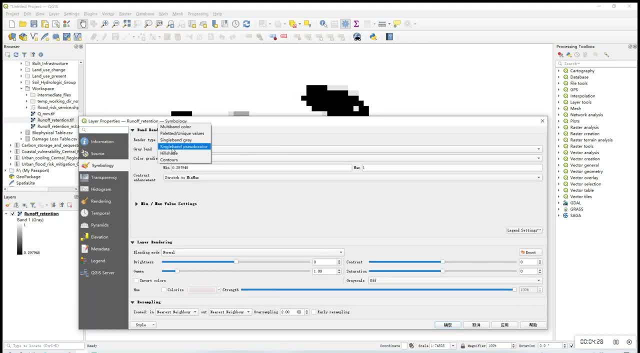 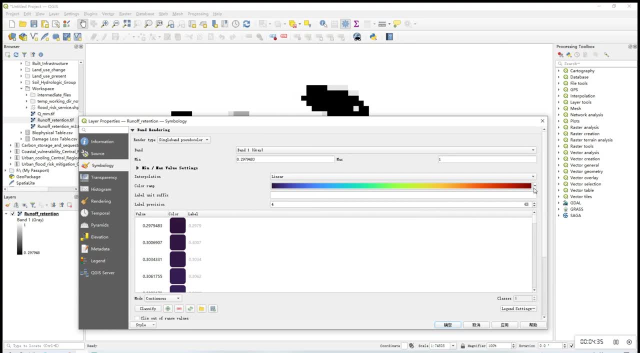 So you can choose to render the images using your preferred color. You can choose the colors from here. You can play around with the colors and apply them to all of your maps, but it would be better to keep the color combination consistent for a given model Once you've rendered all the images.